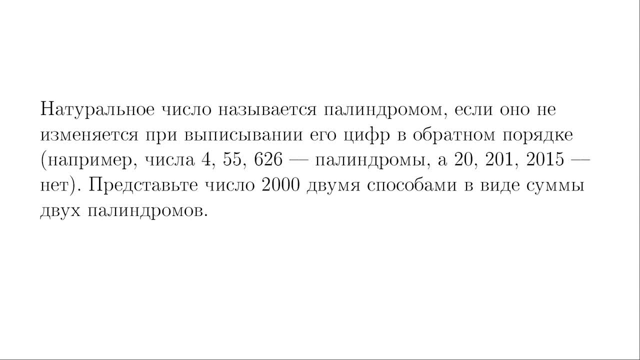 The translation will follow shortly, but first let's get you the daily dosage of Russian you didn't know you needed. Представьте число 2000 двумя способами, в виде суммы двух палиндромов. 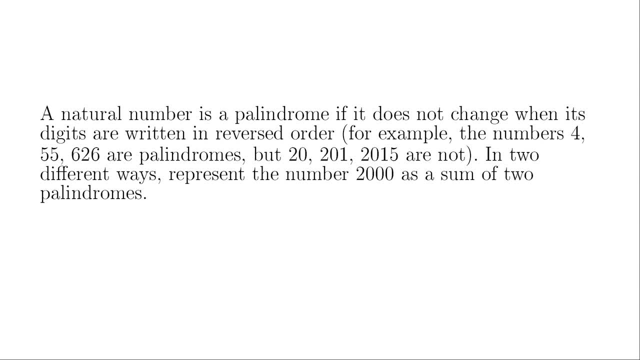 And now the English version. A natural number is a palindrome if it doesn't change when its digits are written in reversed order. For example, the numbers 4,, 55, 626 are palindromes, but 20,, 201, 2015 are not. 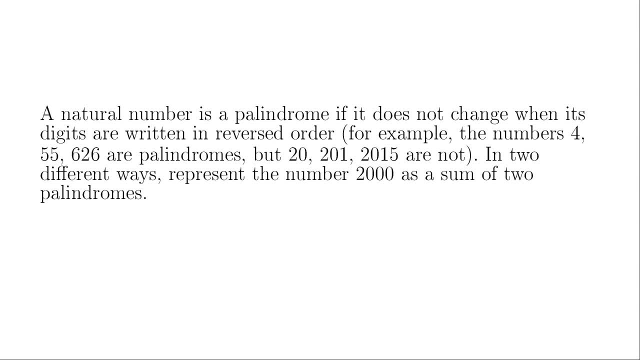 In two different ways represent the number 2000 as a sum of two palindromes. I will now give you a couple of seconds to pause the video in case you want to first try and solve the problem yourself. First we realize that one of the numbers in the sum has four digits Otherwise, 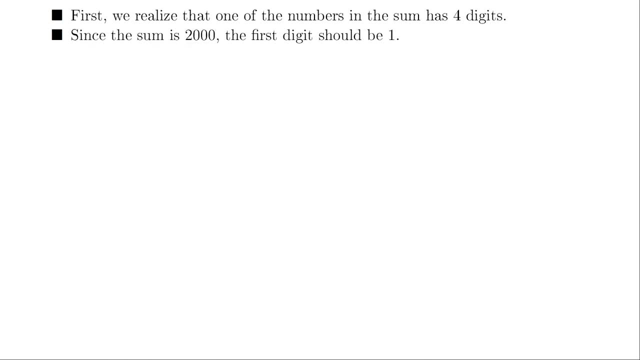 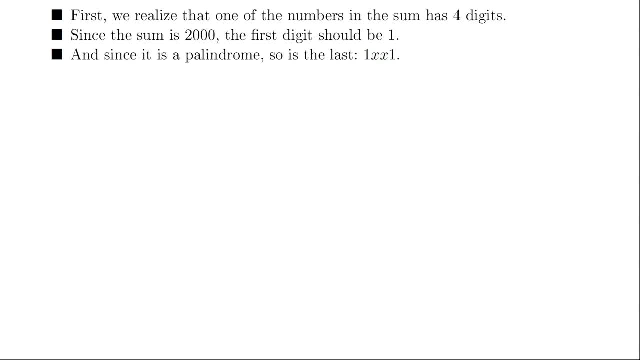 the first digit has to be one, And since it's a palindrome, the first digit has to be one, And since it's a palindrome, so is the last meaning that we can represent our number as 1xx1,, where x is unknown. 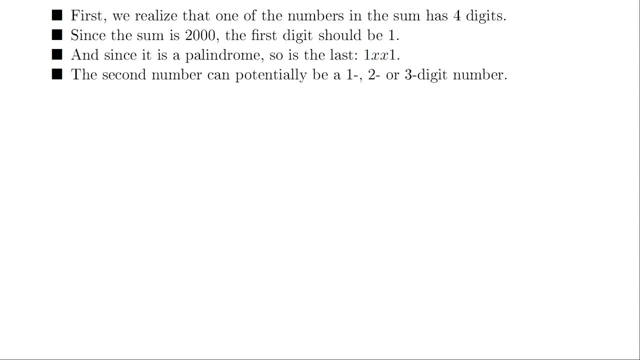 The second number can potentially be a 1,, 2 or 3 digit number. Since its sum with 1xx1 should give a zero in the ones, its last number is 9.. And since it's a palindrome, so is the first. We have three alternatives: 9,, 99,. 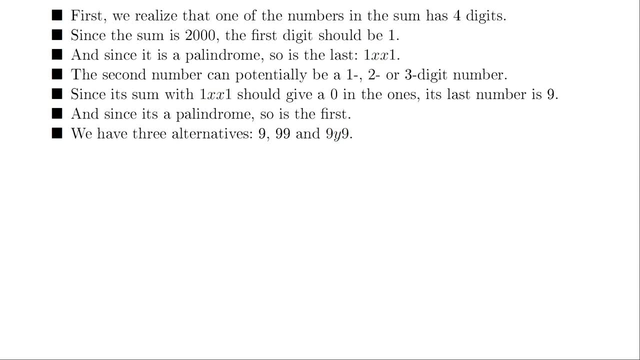 and 9, y9, where y is unknown. For 9, we have 2000 minus 1,, equals to 1,991, a palindrome. For 99, we have 2000 minus 99, equals to 1,901,, which is not a palindrome.